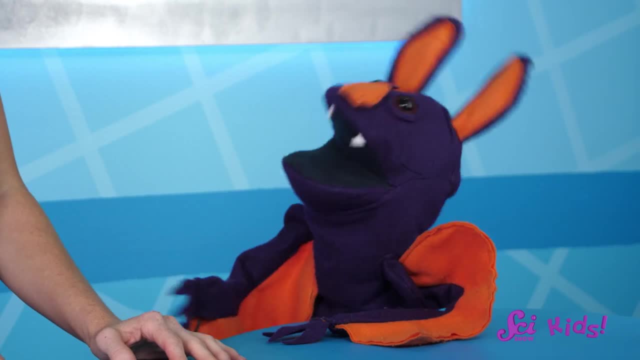 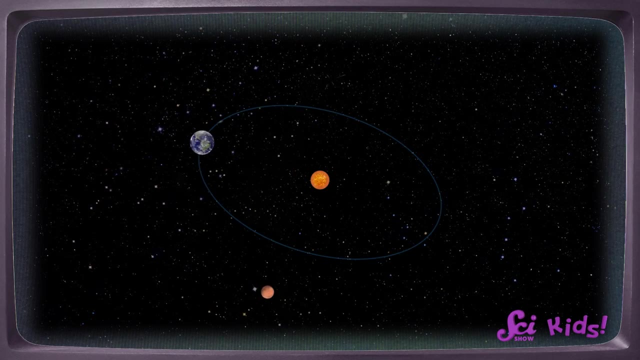 which looks like a man pouring water. Hey, Jessie, do you know why you can't see all the constellations all the time? Ooh, that is a great question, Sam. The Earth moves around our Sun in a big loop throughout the year. 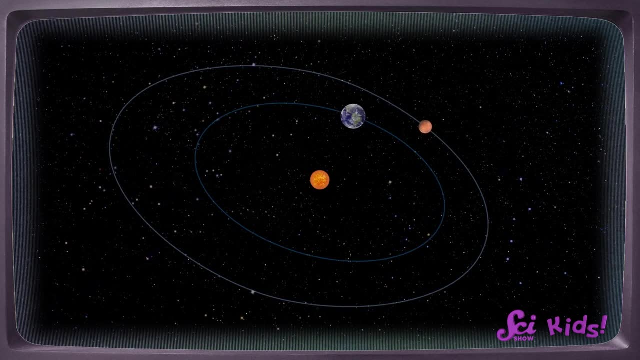 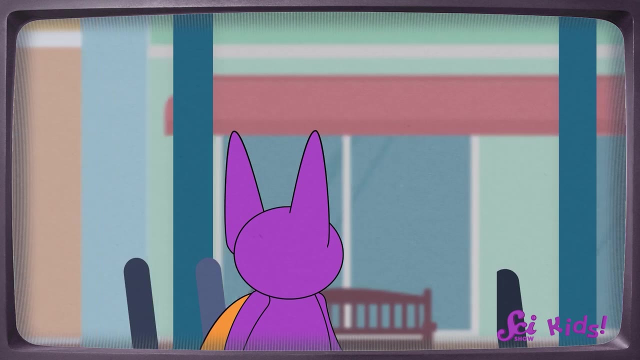 As that happens, we get the chance to look at different parts of space. It's like when you're driving around the block in a car or a bus. As you look out the window, you get to see different buildings that seem to move past you. 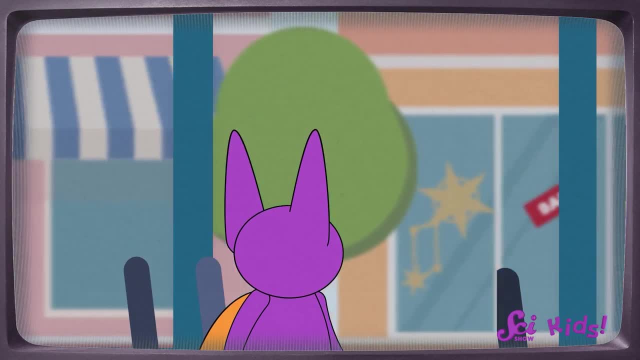 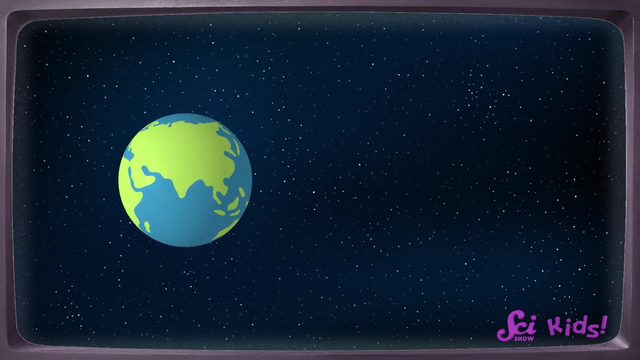 Because you're moving, you get a different view of the space around you, even though the buildings out there are actually staying still. Earth is like our bus and all of the stars and constellations stay in the same place, But we move and see different ones throughout the year. 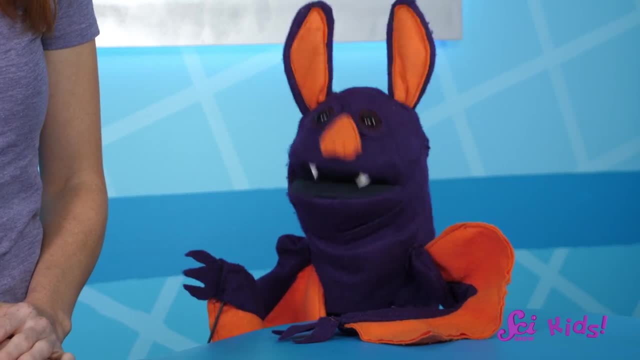 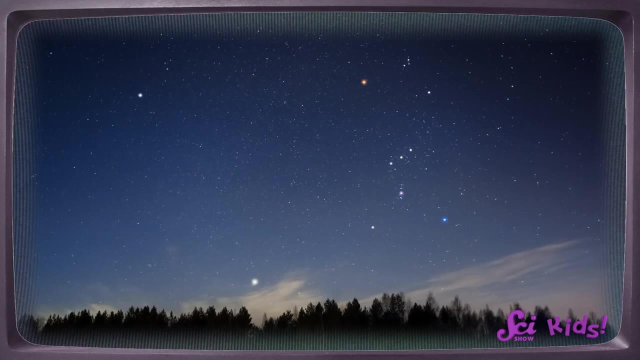 Yeah, and what part of space you can see changes depending on what time of year it is. As the Earth moves around the Sun, we have a different view of space, so we can see different stars and constellations, Like I've been looking at the constellation Orion. 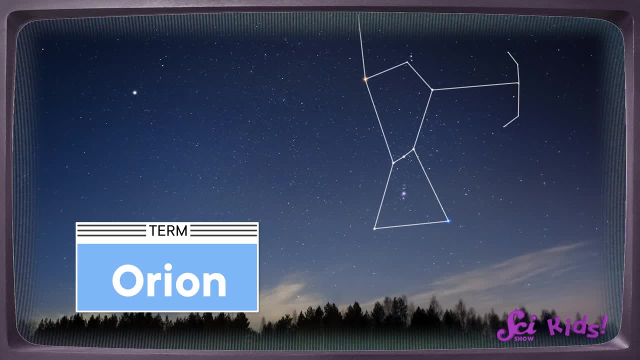 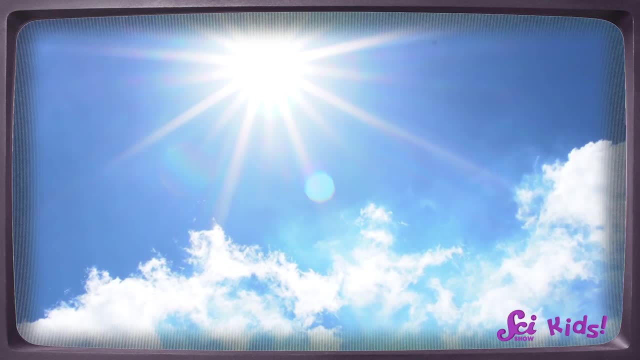 Orion is easy to see from November to February here in the Northern Hemisphere because we're facing it at nighttime. But by June our planet has moved to a place where we're facing Orion during the daytime and the Sun is too bright for us to see it then. 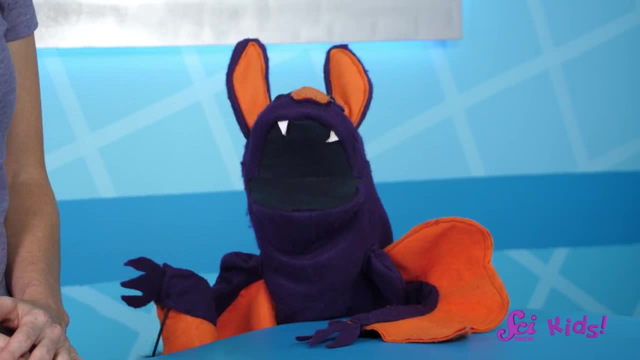 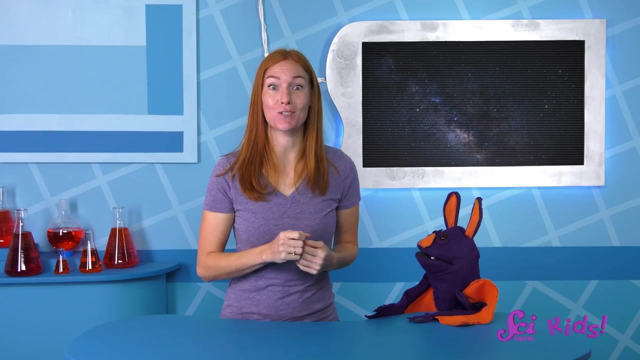 So at night Orion is completely out of view and we see other stars. Constellations are so fascinating, And these star pictures aren't just for fun. Some stars and the constellations that help us recognize them are really important for helping people find their way. 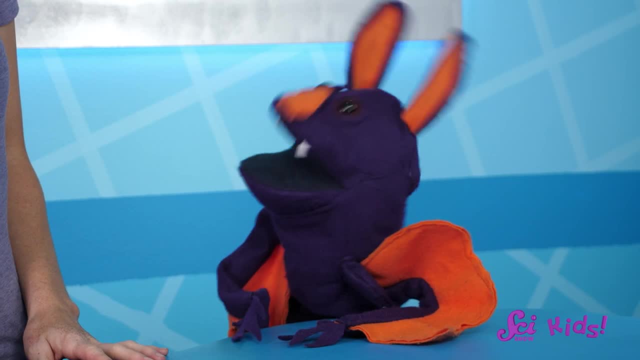 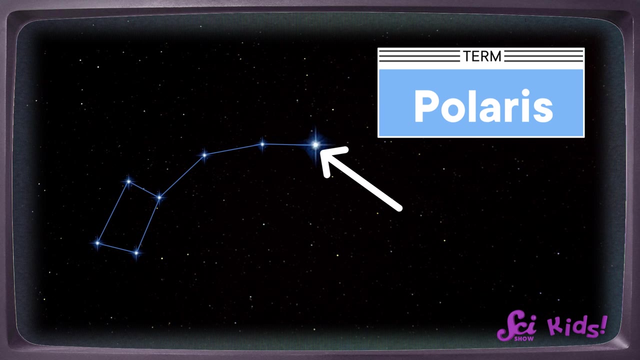 That's so cool, But how can a star help someone find their way? Let me show you. This is Polaris, the brightest star in the constellation Ursa Minor. Some people call Ursa Minor the Little Bear or the Little Dipper. 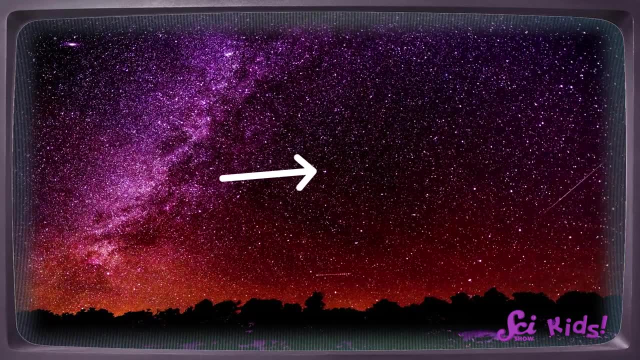 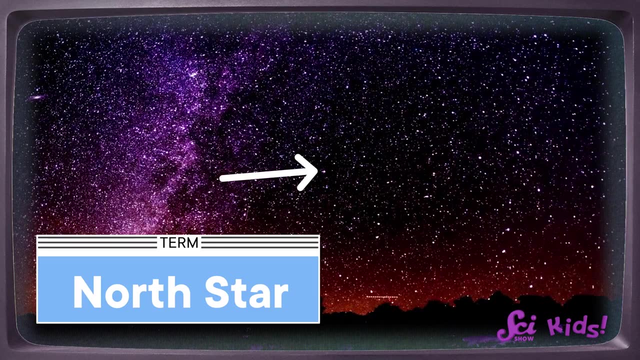 Oh, I know about Polaris. It has another name too. Some people call it the North Star. That's right. When we look up into the sky, the North Star is always north of us. That means that if you can find the North Star, you know how to go north. 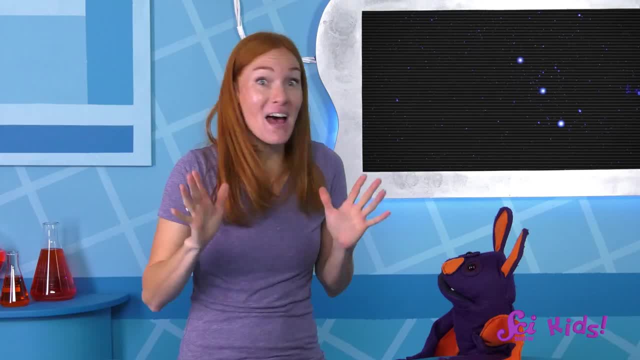 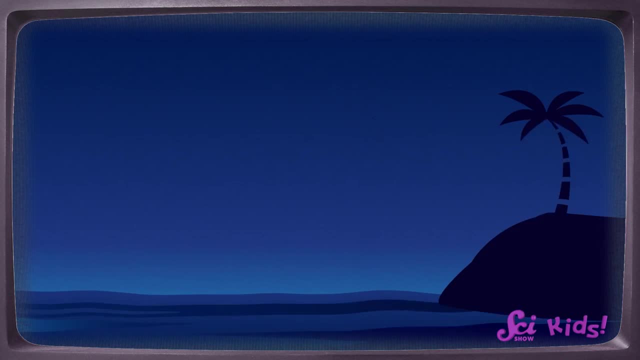 But what if you don't need to go north? What if you need to go a different direction? That's a good question. Let's say there's a ship full of people who need to get to an island that they know is south of where they are. 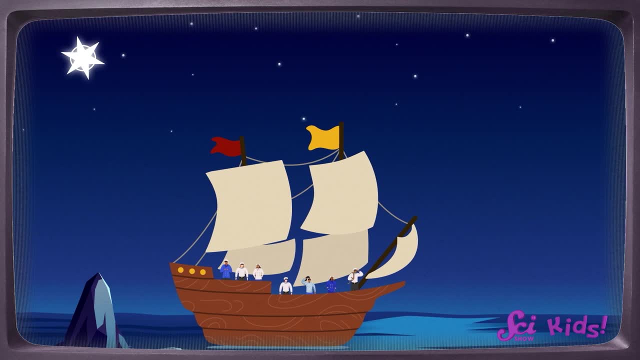 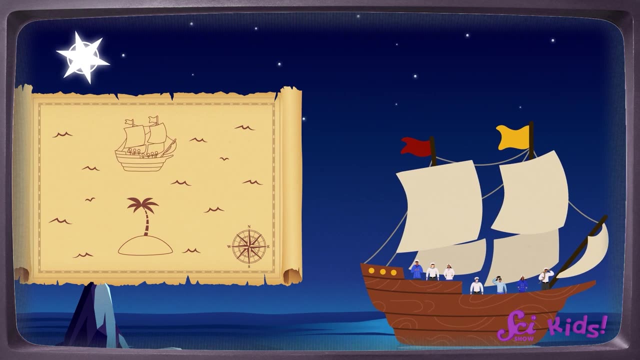 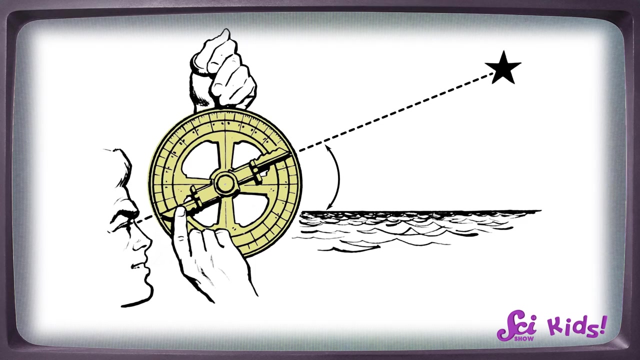 If they look up and find the North Star, they just need to sail in the opposite direction of that star, Even if they have a map to tell them where to go. they can always check Polaris to make sure they're on track. And as people got better at navigating and finding their way with the stars they designed, 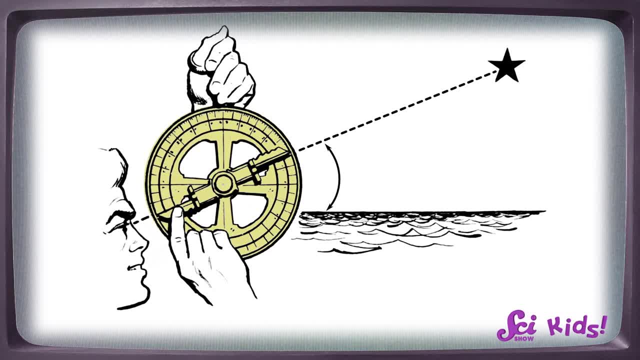 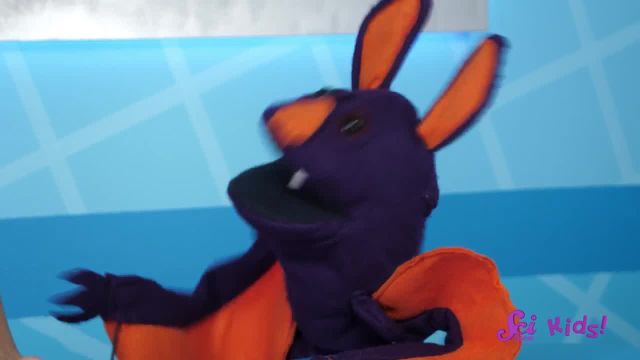 special tools that help them. use Polaris to guide them even across the ocean. It's amazing that a star can be so helpful even though it's super far away. Ooh hey, Jessie, do you want to look and see if we can find a bat-shaped constellation? 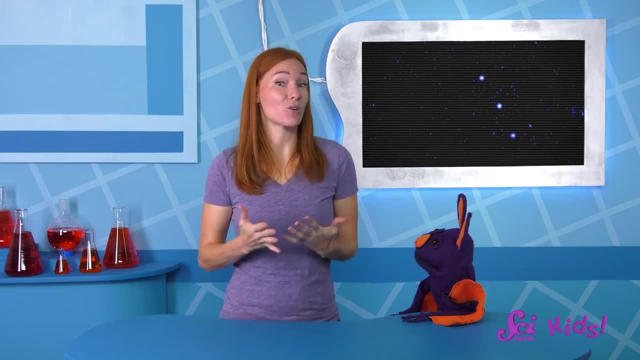 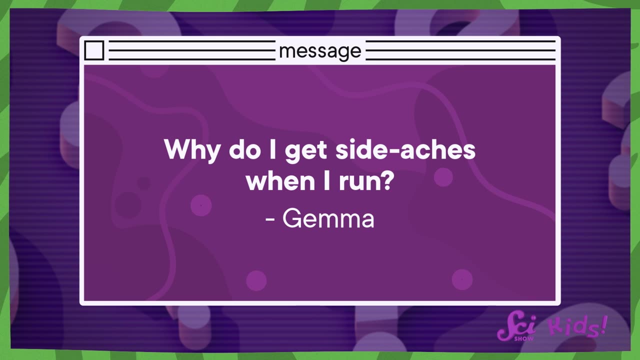 We can certainly try Before we go. do you want to answer a question from one of our viewers? Sure, that sounds fun. Okay, today's question comes from Gemma, age 8.. Gemma asks: Why do I get side aches when I run? 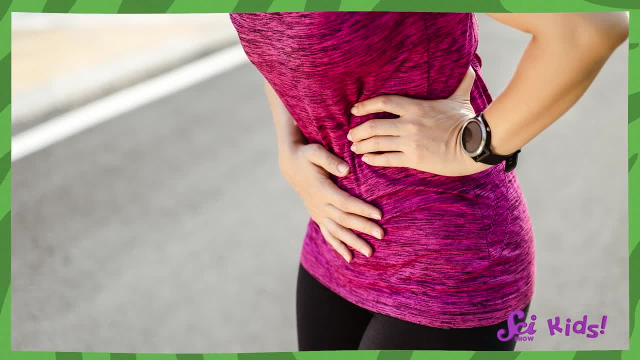 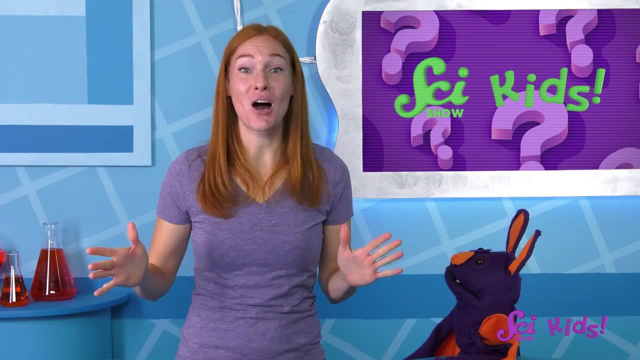 Well, side aches or side stitches are common for many people when they run, swim and exercise. Side stitches can hurt like you've pulled a muscle in your side. Doctors don't actually know for certain what causes them yet, but scientists have some ideas. 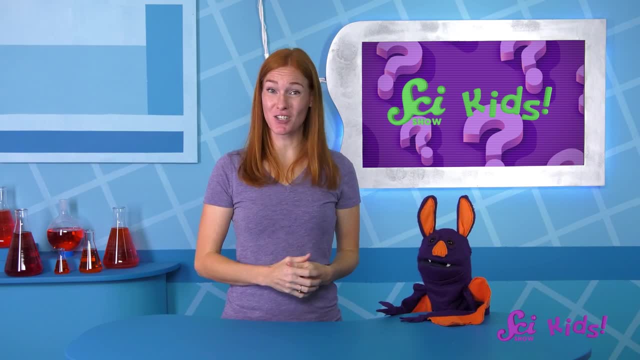 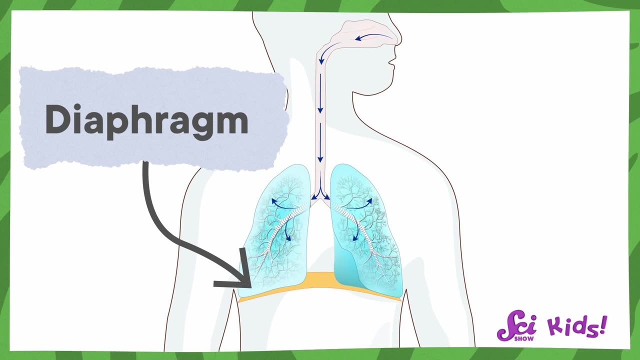 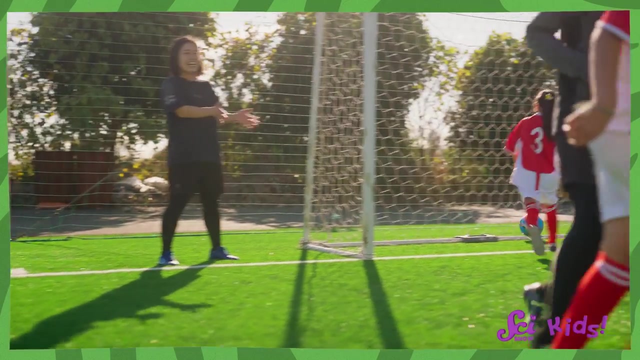 There are a few body parts near where people feel side stitches that could be causing the pain. First, it could be your diaphragm. The diaphragm is a special muscle under your lungs that helps with breathing. When you run, you have to breathe more heavily and your diaphragm has to work harder. 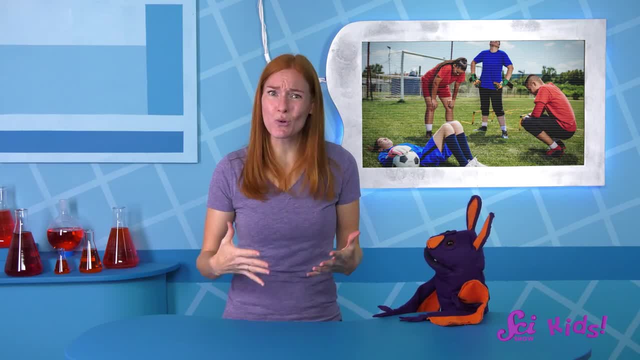 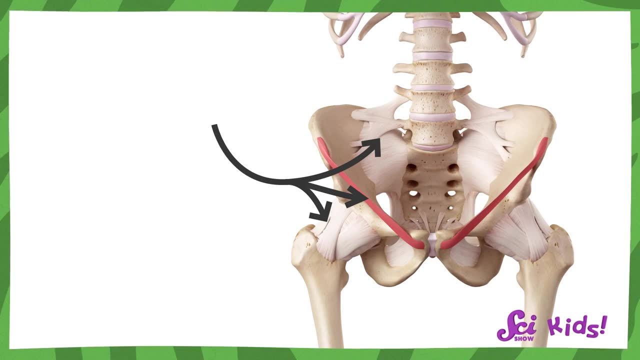 Side aches could be caused by your diaphragm getting sore from working so hard. Another idea is that the pain could come from the ligaments near your diaphragm. Ligaments are special body parts inside that help hold your body parts together. 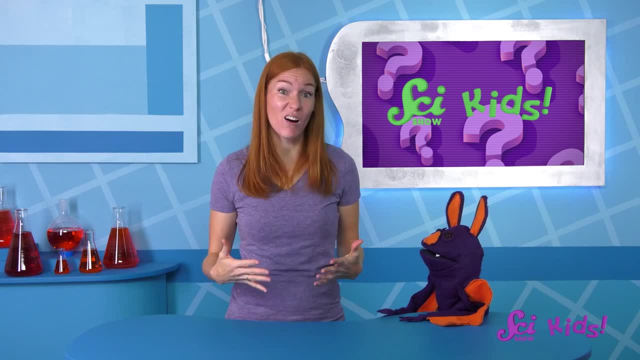 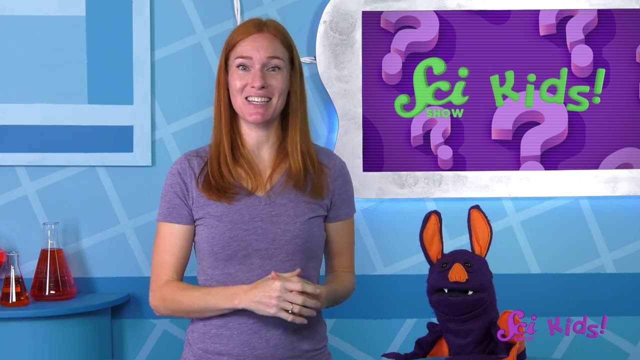 If the ligaments get jolted around and aren't used to working hard to hold things together while you run, they could get sore too. So what do you think? Let us know in the comments If you don't yet know exactly what causes side stitches. doctors do know some ways to help avoid them. You could wait a little while after you eat before you go run and play, instead of getting up right after, And make sure to stretch your sides and your middle before doing a lot of running around. 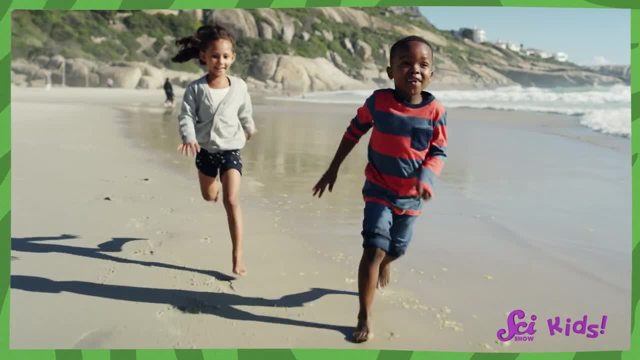 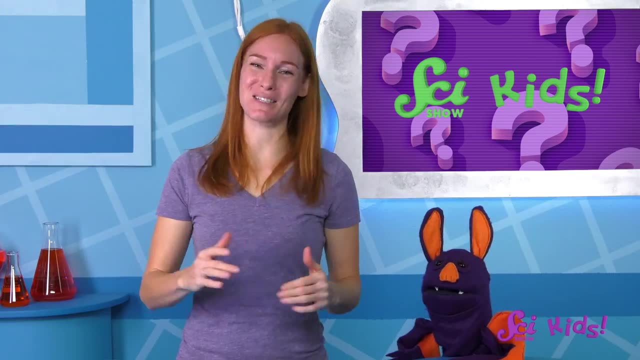 And keep growing stronger. As you practice things like running more, your muscles and ligaments can grow stronger and won't get tired and sore as easily. Thank you for your awesome question, Gemma, and good luck with your running. Meanwhile, I think we'll exercise our